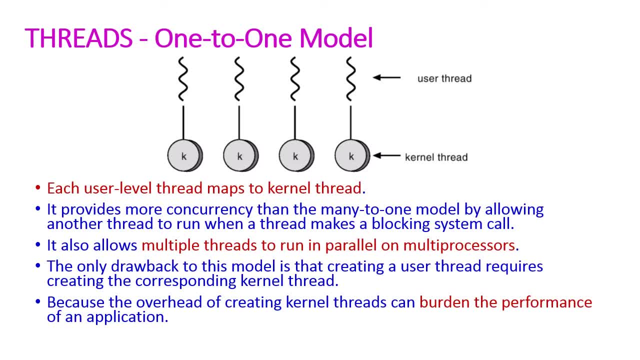 To overcome the drawback of many to one model, here we are having one to one model, One to one thread model. Here each user level thread maps with the corresponding kernel level thread. Here we are having four user level thread For all the four threads we are having. 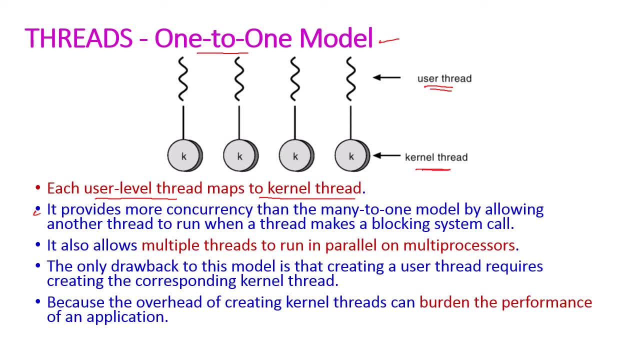 separate kernel thread. Okay. hence it provides more concurrency than many to one model, and this model will allow the threads to run. even the system blocking system call occurs because the operating system calls. So this is the very big drawback of many to one model: Here, each user. 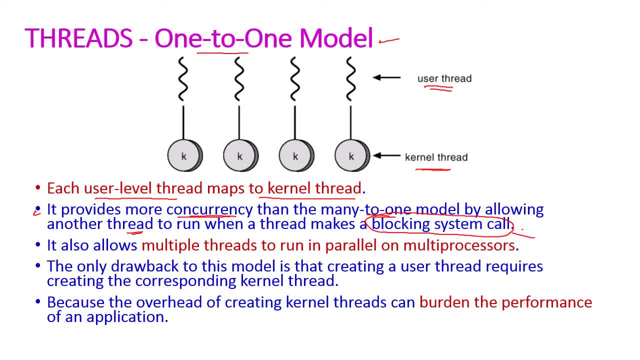 system will allocate the separate or another thread call to take care of this blocking system call, and it allows multiple threads to run parallel on multi processors. Okay, because for all the user thread we are having corresponding kernel thread, Hence all the threads can run simultaneously. 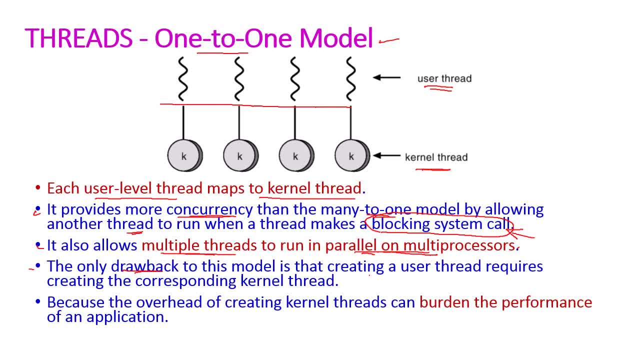 The only drawback of this model is creating a user thread which requires corresponding kernel thread. Okay, for all user threads there should be a same number of kernel thread which overheads the creating kernel thread, and it creates additional burden to the performance of applications. 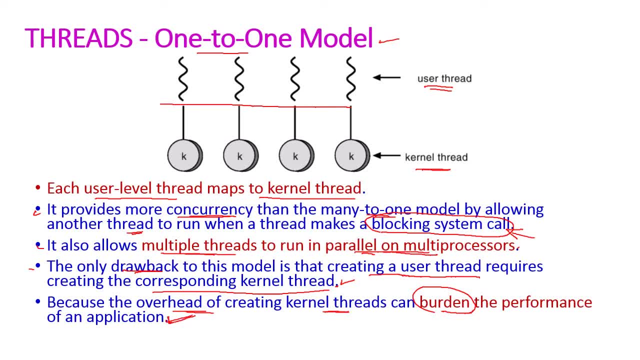 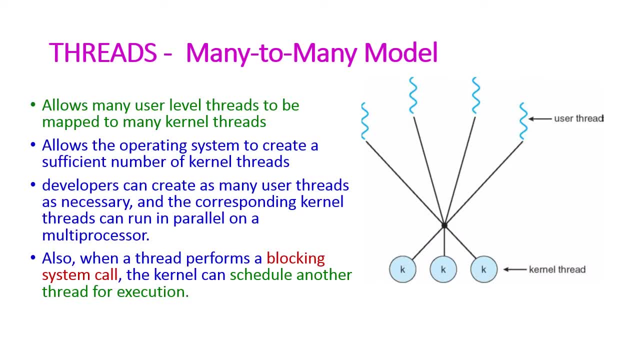 Suppose, if we create more number of kernel level thread, then the burden of operating system will get increased. To overcome the drawback of one to one model, here we are having many to many model, That is, many to one model model. Hence we are having many to many models. 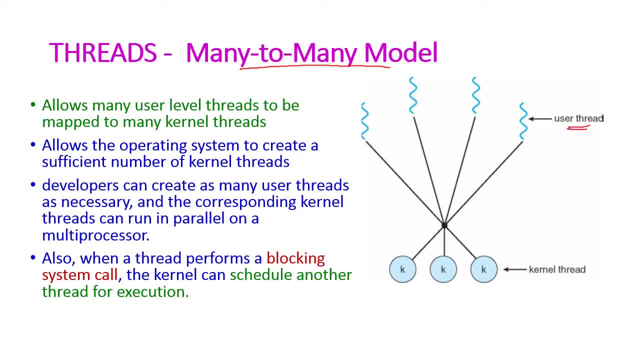 That is, many user level threads will be mapped into many kernel level threads. It allows many user level threads to be mapped with many kernel level threads and also it allows the operating system to create a sufficient number of kernel level threads. Here developer can create many user level threads and the corresponding kernel level thread can run parallel on the multiprocessor system.